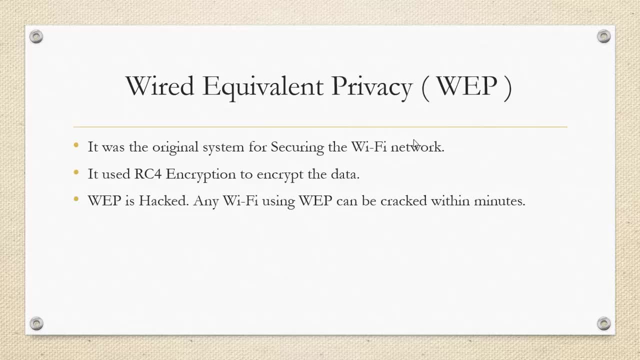 IEEE decided to build much more robust and stronger standard. However, if they would have built a very strong standard, then hardware changes were required, But during that time, lot of people had already bought the web based router. So what they decided to do is they. 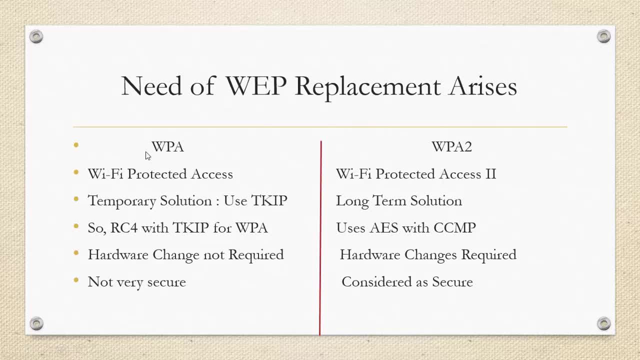 decided to make a temporary solution which was called WPA. One of the advantages of WPA2 was hardware change was not required. However, disadvantage is it is not very secure. WPA2 stands for Wi-Fi- Protected Access, and it was built on top of web. However, it used TKIP. 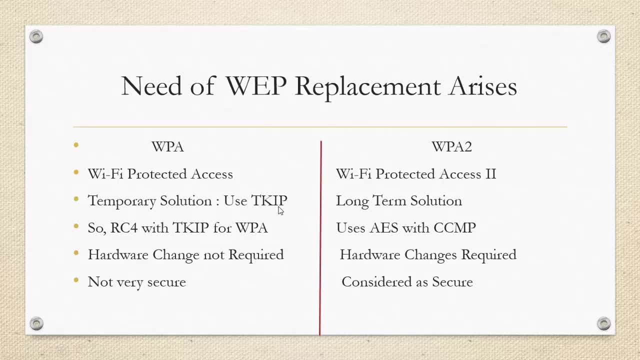 along with the RC4. So the people who were using web-based routers: they just had to upgrade and they would have got WPA. So WPA is still not hacked, but there are a lot of attacks which are targeting WPA nowadays. So, as it was a temporary based solution after WPA, 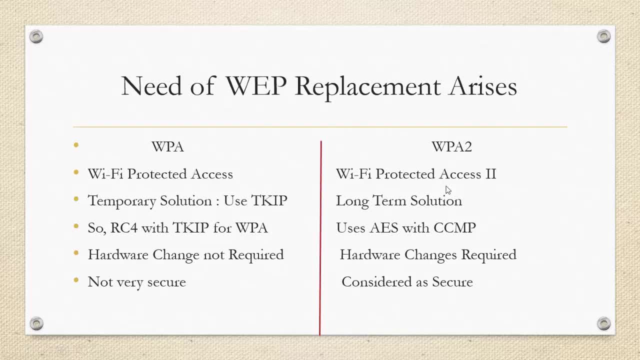 I typically built WPA2, which was a long time solution, and this is what we use in most of the routers nowadays. One of the disadvantages of WPA2 was Hardware change was required. So all the routers during the old times which had web and would need to be changed to support WPA2, so all the new. 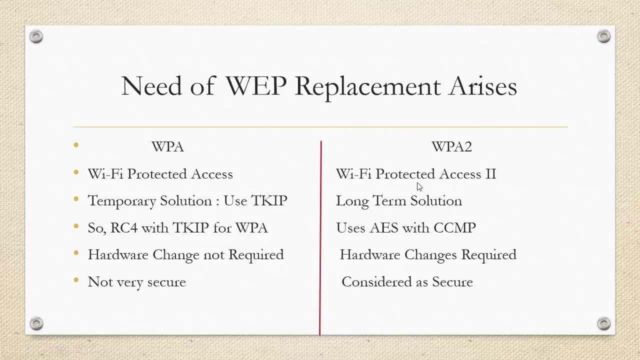 routers was reconfigured with WPA2.. One of the significant changes was WPA2 used AES along with CCMP, So TKIP and RC4 were scrapped and newer and much better encryption algorithm were implemented. It is considered very secure and WPA2 nowadays does not have a proper vulnerability through. 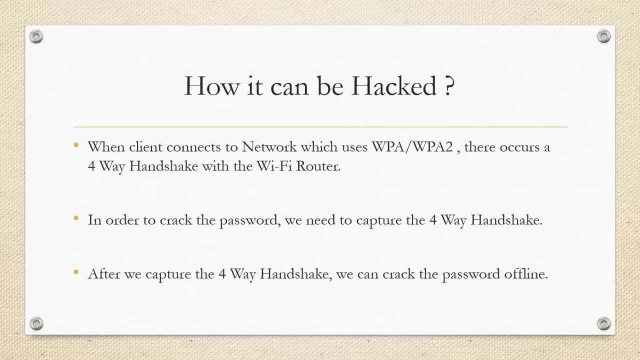 which it can be hacked easily. So one of the ways where WPA2 can be hacked is when a client connects to a Wi-Fi access point which is based on WPA or WPA2, there occurs a four-way handshake with the router.